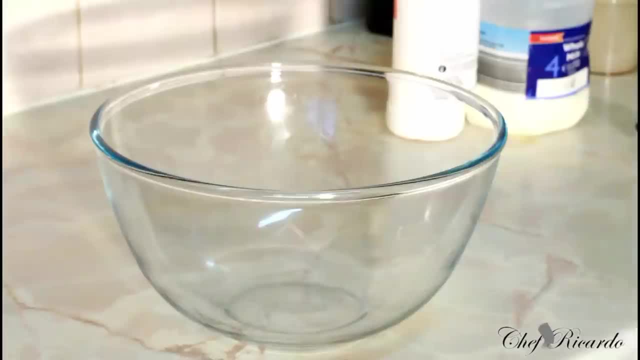 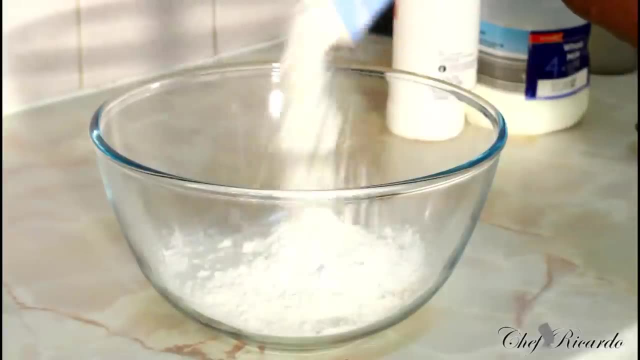 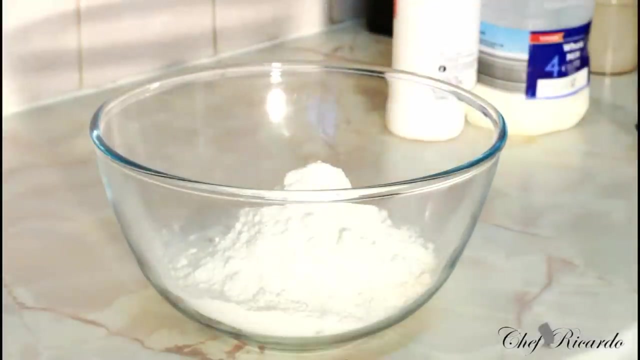 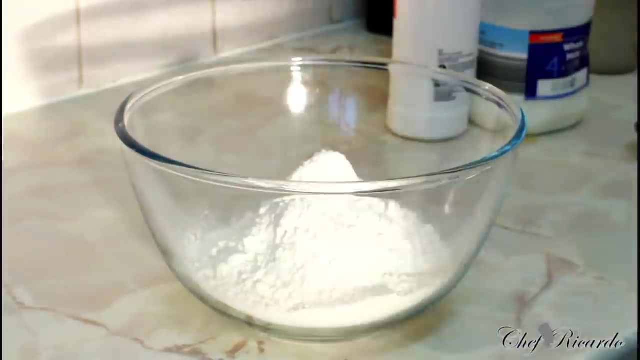 you need a big bowl like this, two cups of self-rising flour. I'm just pouring it from above right here, Roughly Basically. I'm using roughly two and a half cups of self-rising flour, Two and a half cups of self-rising flour inside of this bowl, right here as you. 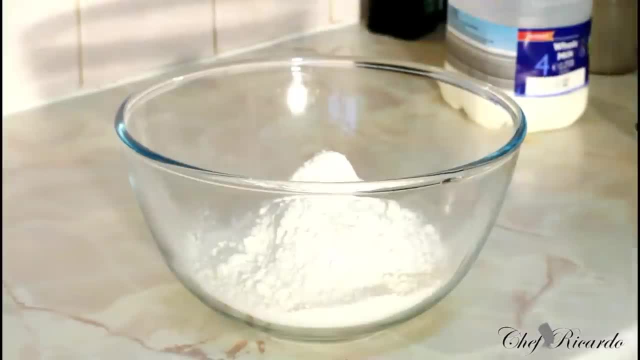 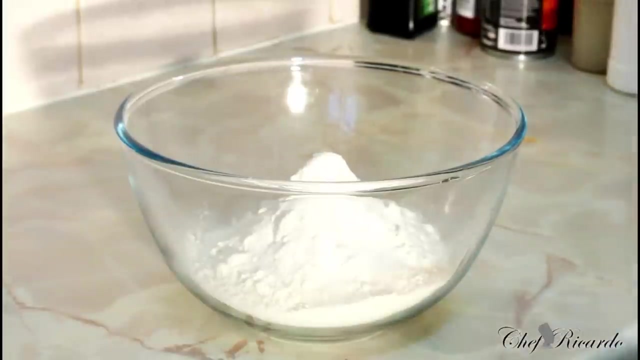 can see, like I did earlier, A pinch of salt, Teaspoon of sugar, And I'm going to use some Ola milk for the mixture. You can use cold ice water or you can use milk. Ola milk, Really really cold, is good for it, alright, So basically, 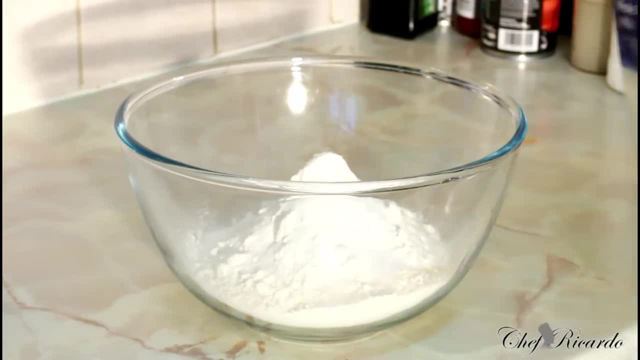 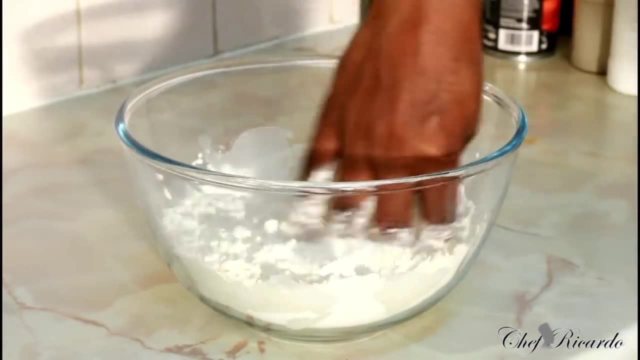 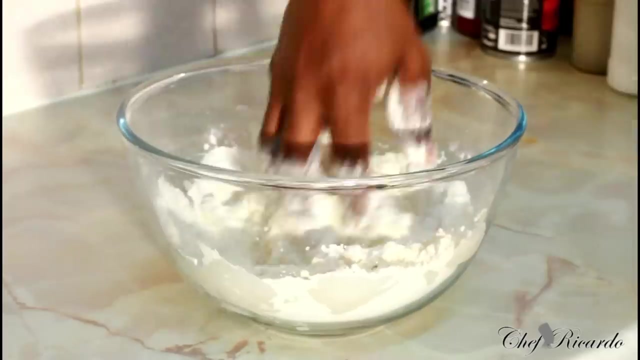 what I'm going to do. I'm going to do a simple: stop, Pour some, Mix it up, just like this, Pour a little bit inside of it. So what you want to do, you want it to form a dough. So, basically, take a look at time And pour tea, Make sure. 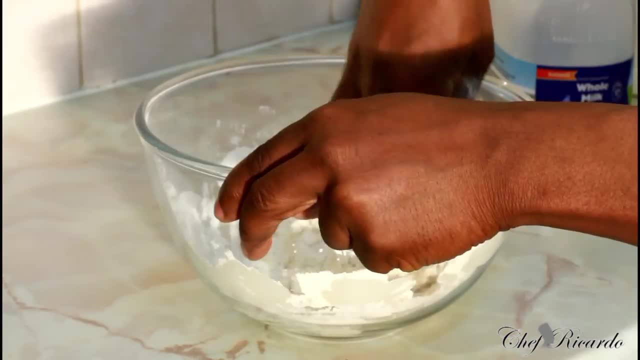 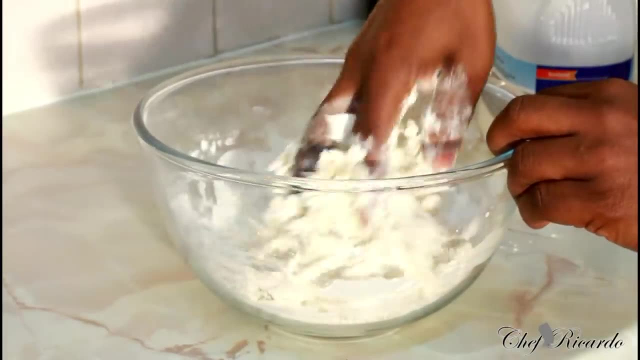 before you start making Jamaican dumplings, hand must always clean, guys. Alright, Some people put butter inside of it, So the butter do give it a flavor, but you know what I mean. you don't want to put it in the ice. Sometime I say to myself: it's too much. you know what? 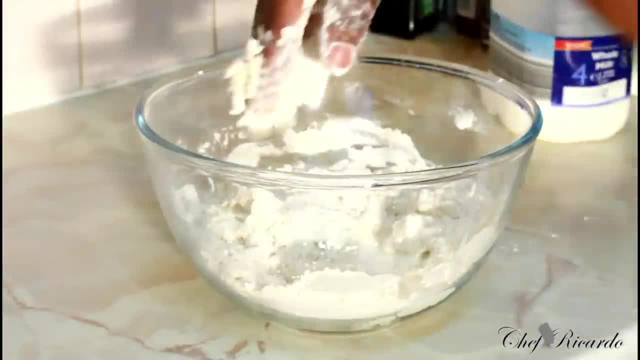 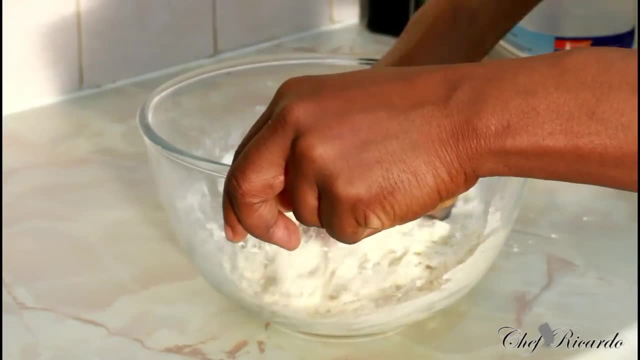 I mean Nice one. As you can see, I'm just continue adding little bit, little bit of milk until you see it form a dough. You don't need, you don't, I don't, you don't need to measure out your. 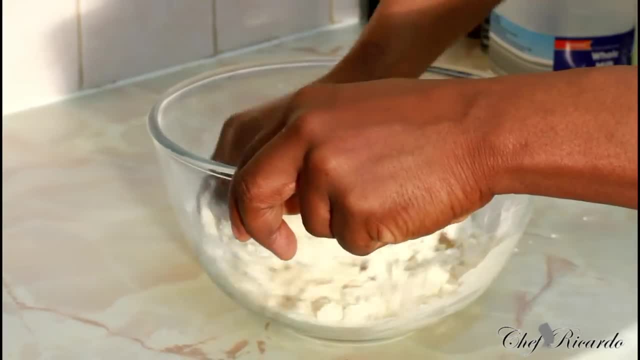 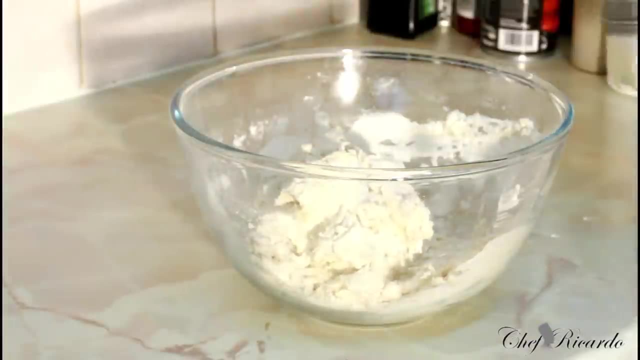 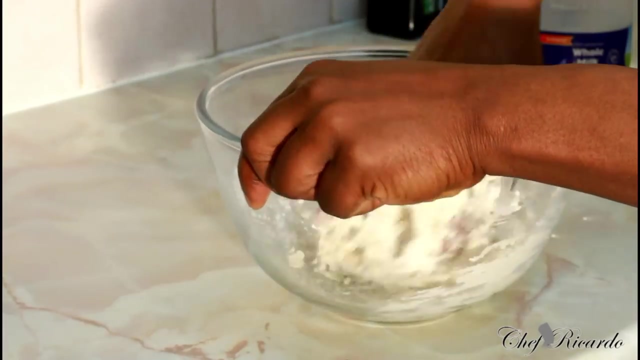 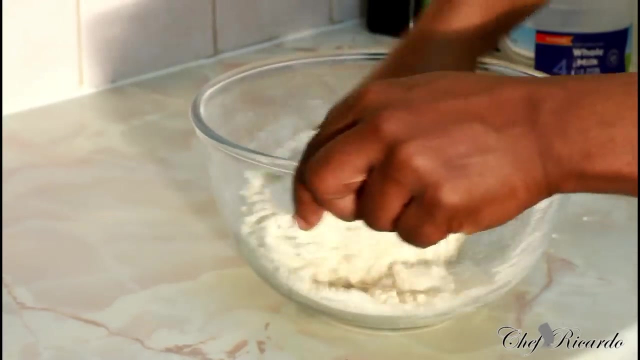 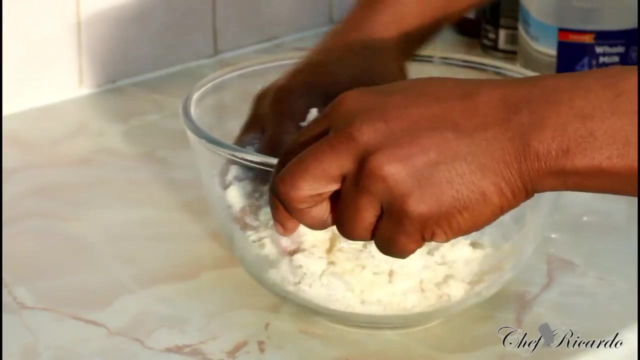 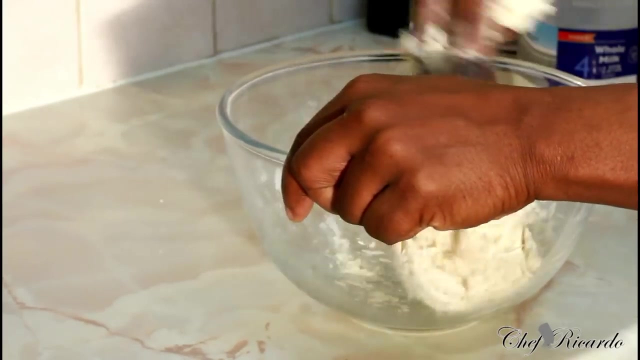 And then I want to. I want to add a little bit more. Some people use plain flour and have baking powder, And some people just use self rising flour, which it's more easier. Add a little bit more 3apt. 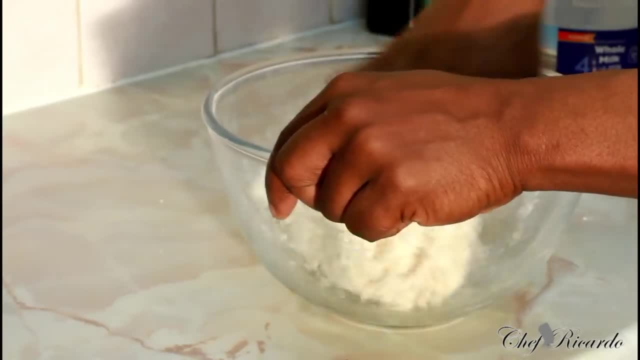 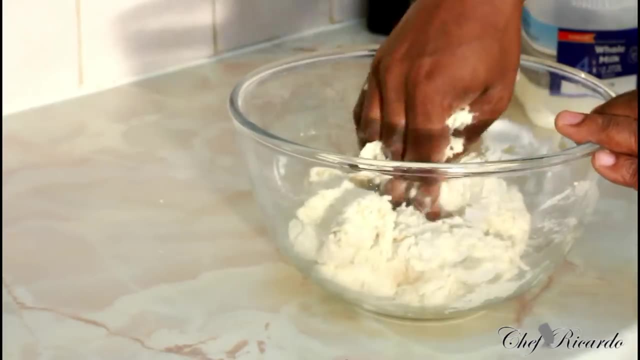 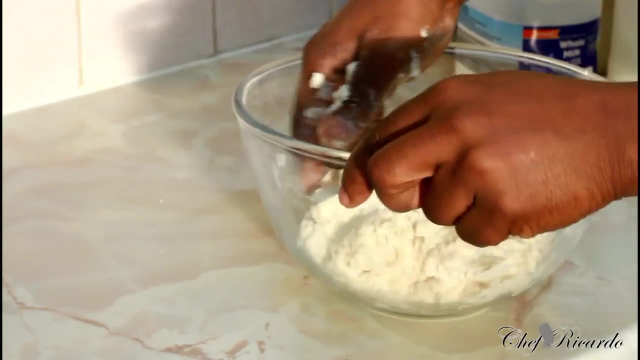 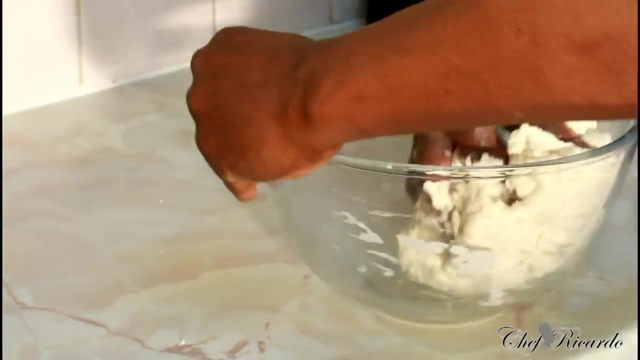 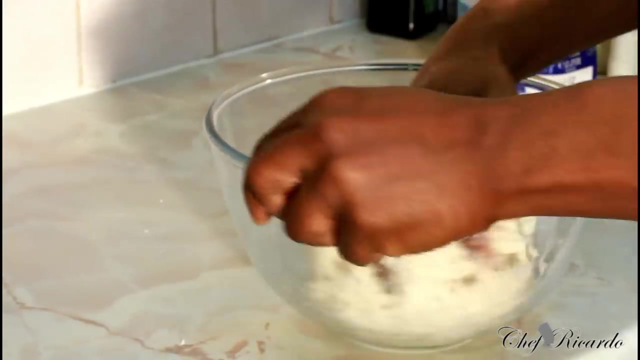 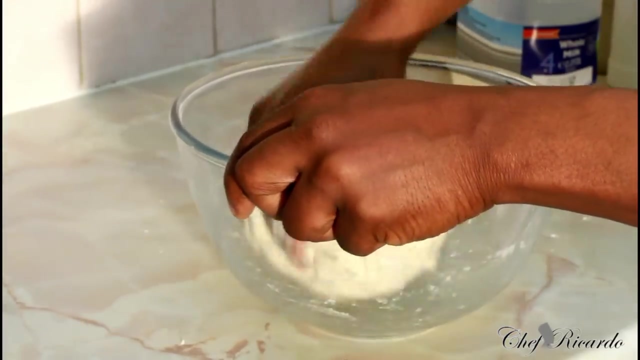 3apt, 3apt, 3apt, 3apt, 3apt. so what? all I need to do is just to get the dough firm together, that's all. so, basically, I'm just gonna out, pop just a little pinch more, use the dough and clean out the board. so basically, as I can see, exactly which I'm all about with. 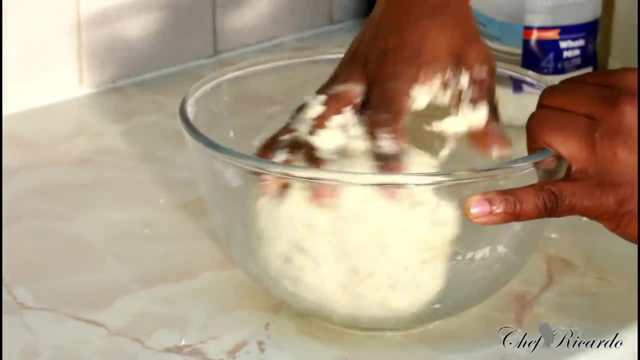 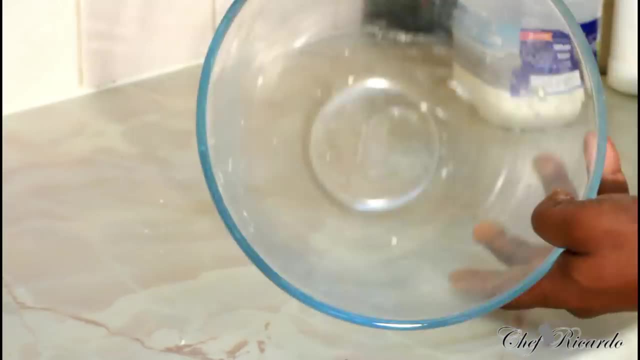 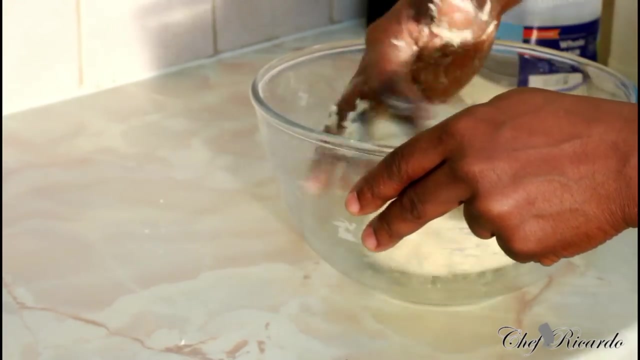 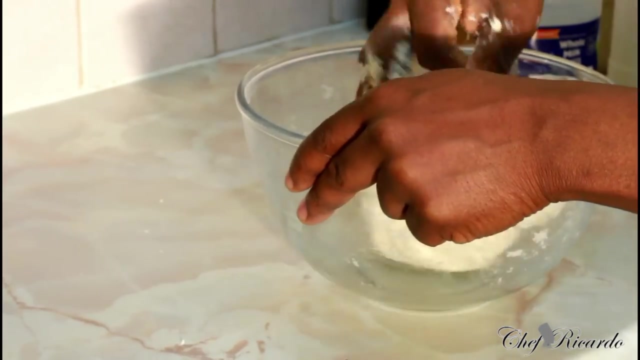 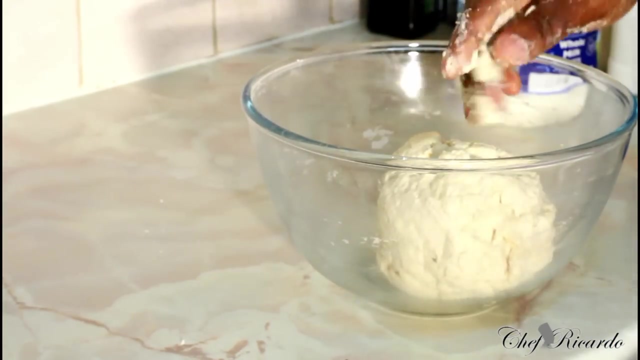 this dough. so basically, as I see it, form the dough like this. this is really good guys. seriously, when you make the dough, it's a supposed to look like this inside, so you want to give it a nice lovely. so, as I can see. remember, as I say, two and a half cups of plain self rising flour. add a. 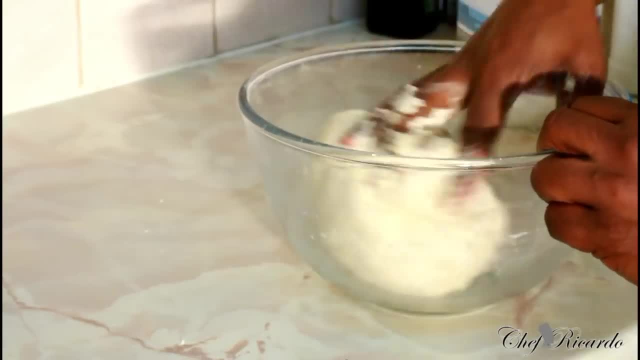 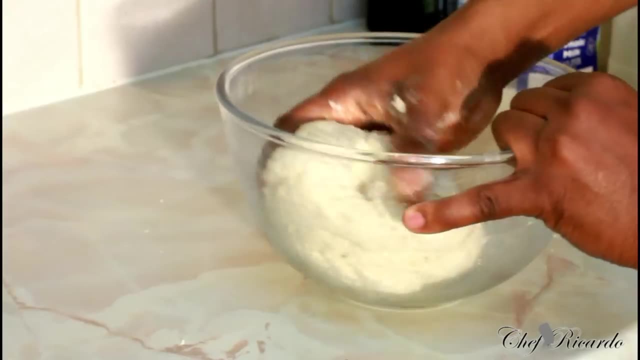 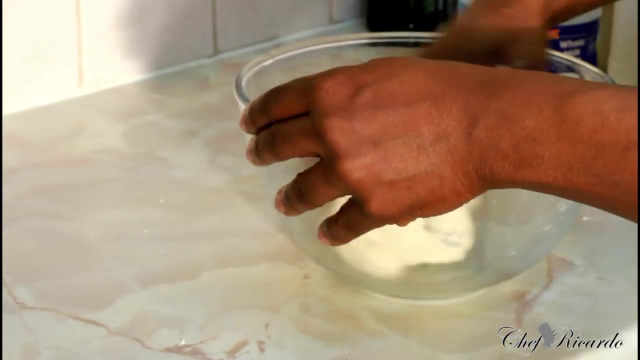 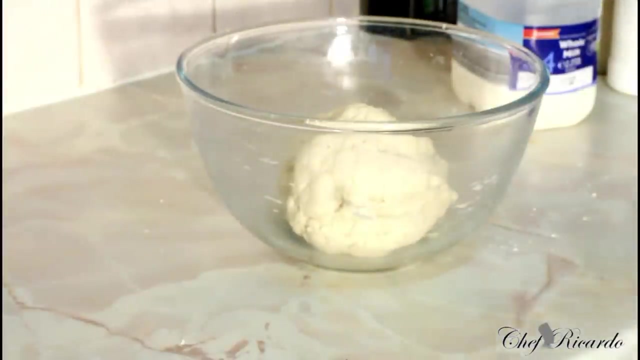 little bit of milk until it form a dough like this. if it is spoiled you can add a little bit more flour to it if it's too soft for you. but it's good to the second at the time. and hard milk, nice and lovely. the next thing we're gonna get the claim flame. 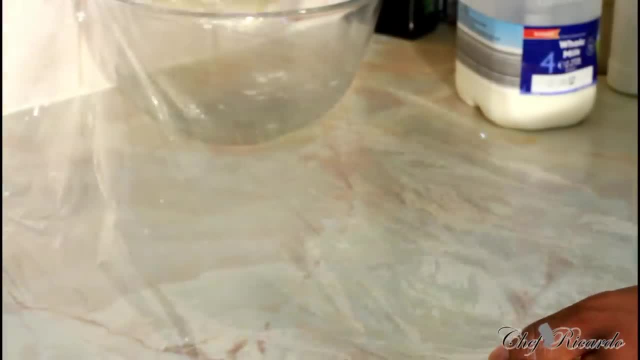 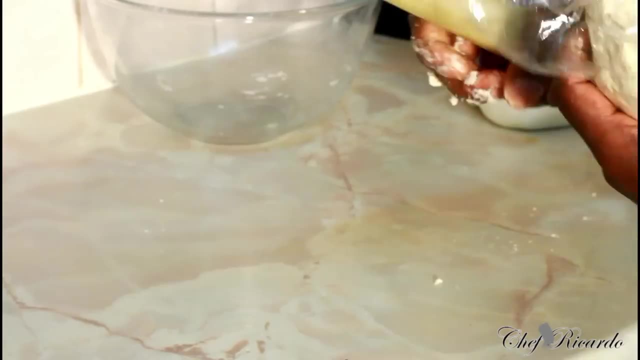 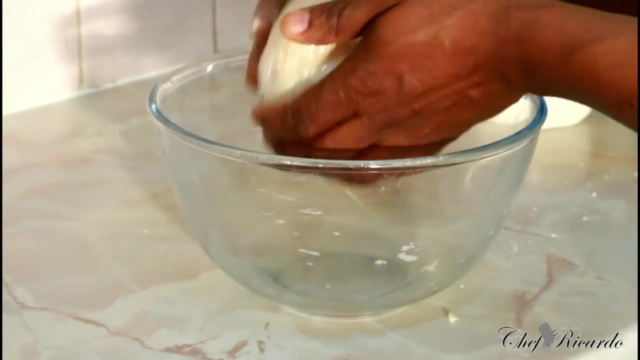 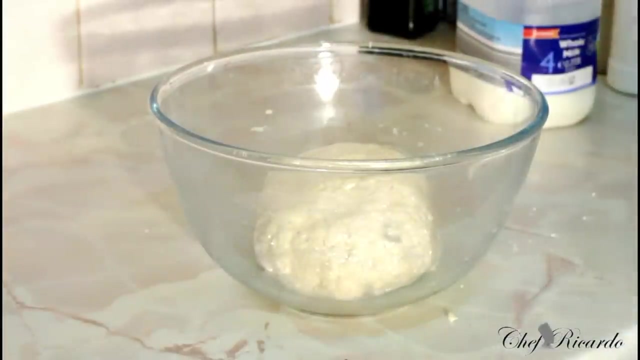 get it like this at this, And leave it inside of the bowl for roughly about half, about 20 minutes, 30 minutes, just to make it get proof and dust. When you make dumpling and you put it to rest like this, guys, it is 100% better and you. 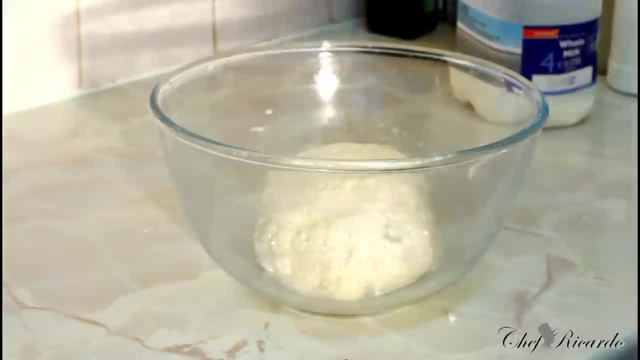 will see the difference when I finish with it. So what you can do, you can simply pop it in the fridge. I just pop it at the surface and today we are ready to start making some dumplings. all right, Enjoy the recipe. 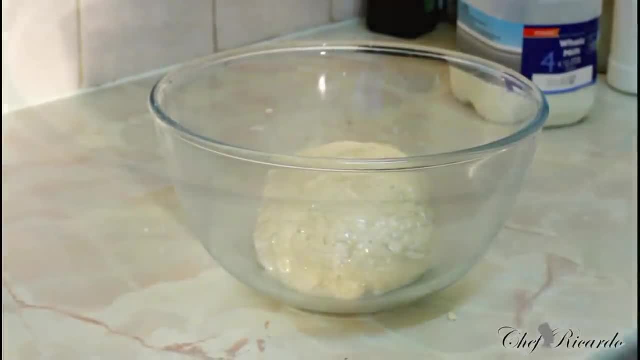 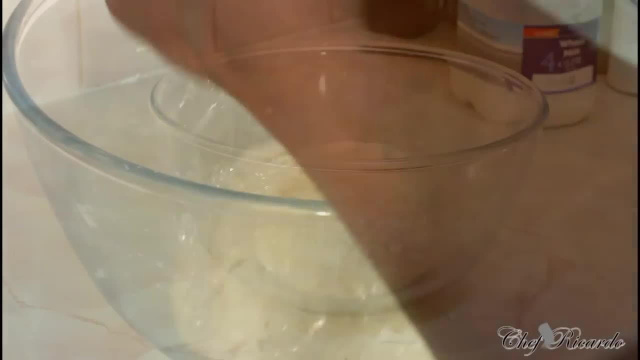 Thank you so much, guys, for watching the cooking show. So, basically what we are going to do, we are going to show you what is going on right here. Remove the cling film from it. you see how the dough is swollen up like puffed up. 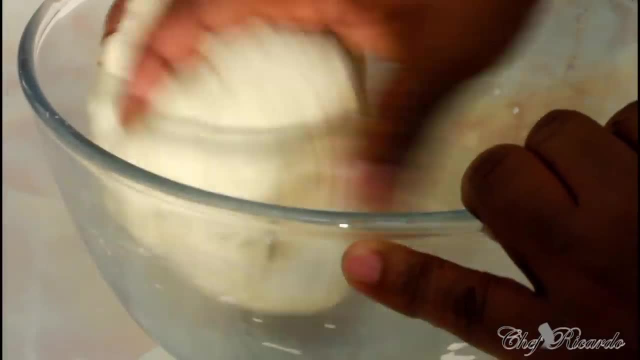 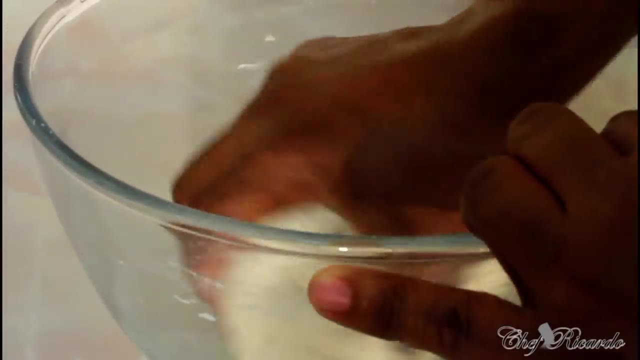 So, as you can see, it even feels a little bit different. so all you have to do is just use your hand And simply work it in, just like this. So I will say, I will give you an idea every time you make a dough for your dumpling, just. 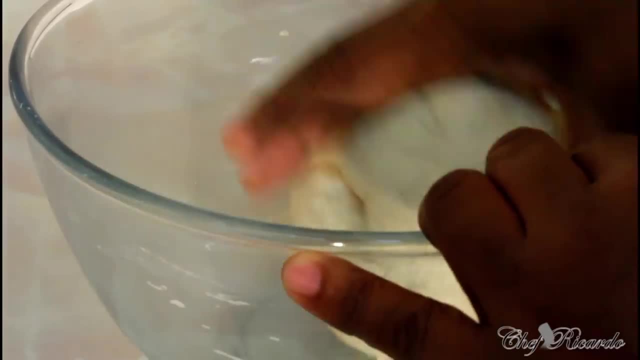 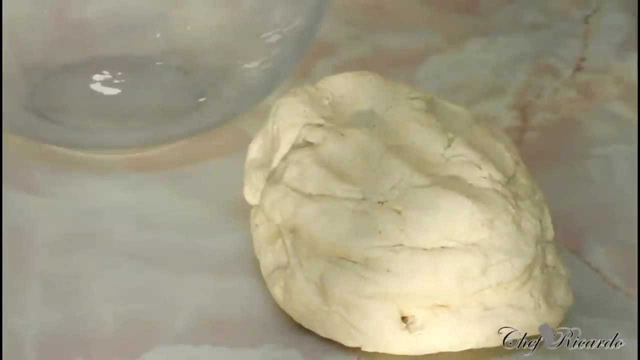 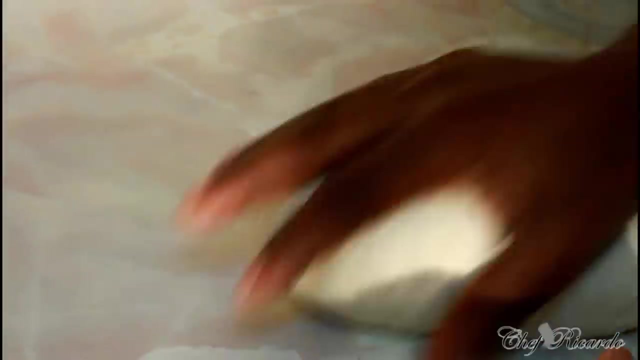 simply wrap it up and put it up for a nice good 20 to 30 minutes, lovely. So just look at that dough, beautiful, the feeling and the texture. So basically, as you can see, looking, feel different, nothing coming off of it. 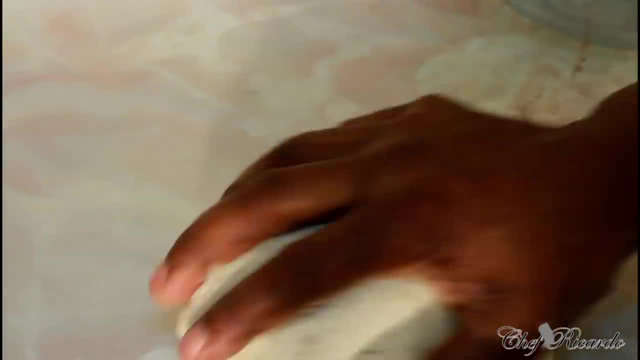 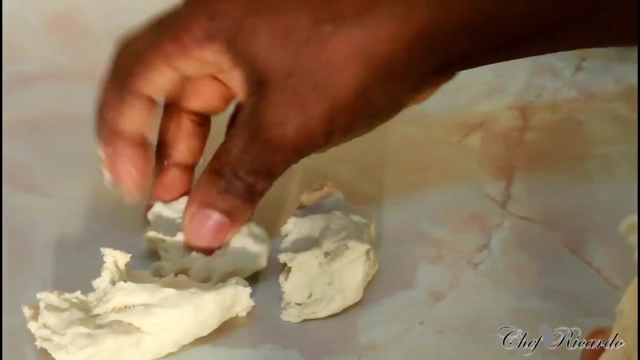 It just flows, It just feels so lovely and nice. So basically what we are going to do, basically. normally, this is how we do it in Jamaica: you break off some little pieces like this to make a dumpling, So I am going to put them back inside of the bowl. 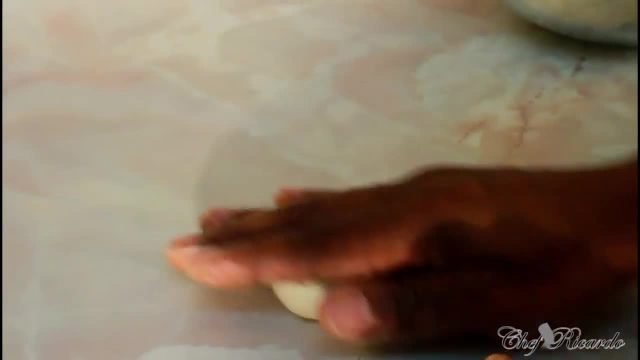 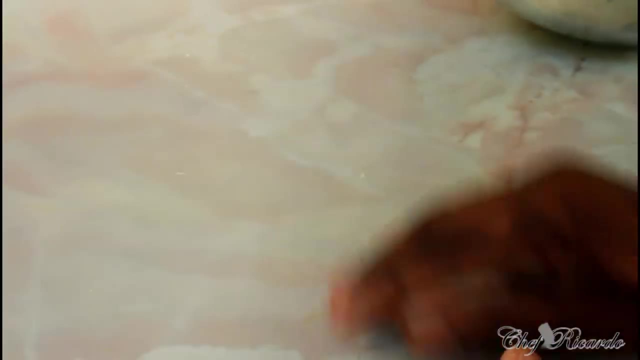 So what we are going to do now? I am not going to make my dumplings massive, so I am going to make them small. In Jamaica, we normally roll it on a surface like this, and this is the way it will come out when you roll it on a working surface just like this. 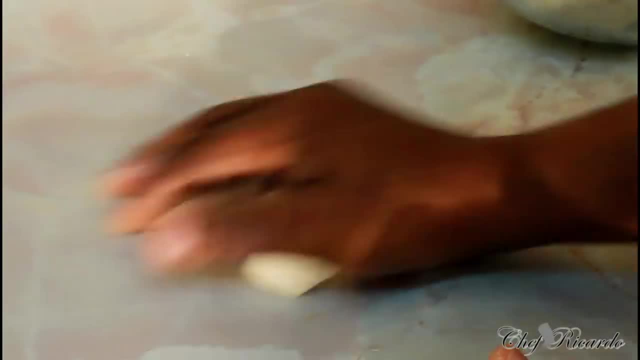 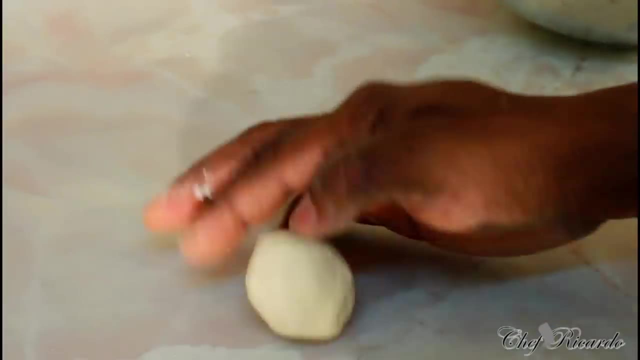 Like this: Lovely and nice. so it comes out really smooth, lovely and nice, especially if you are making mini dumplings. this is the best way to do it. alright, There is another way you can do it if you don't know how to do it. 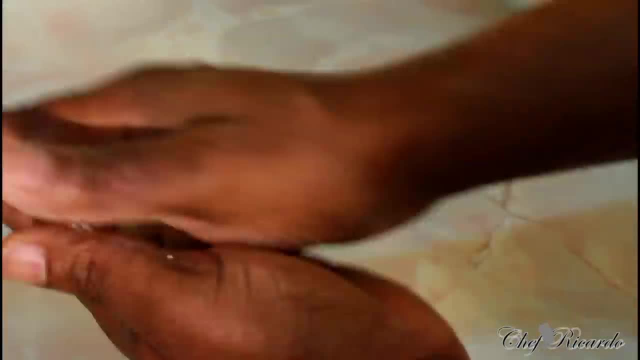 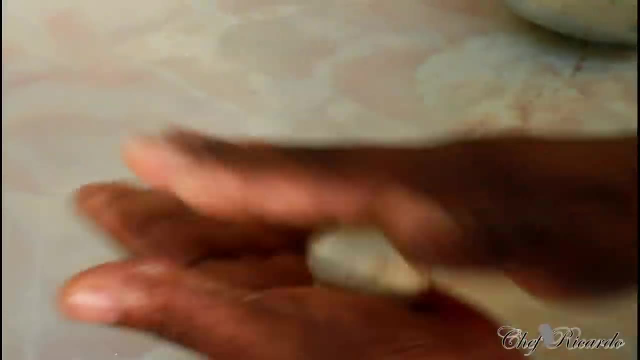 Some people roll it up in their hand like this, But when you roll it in your hand it won't come out so nicely like the one you do on a working surface. That is another way. There is another way you can also do it. 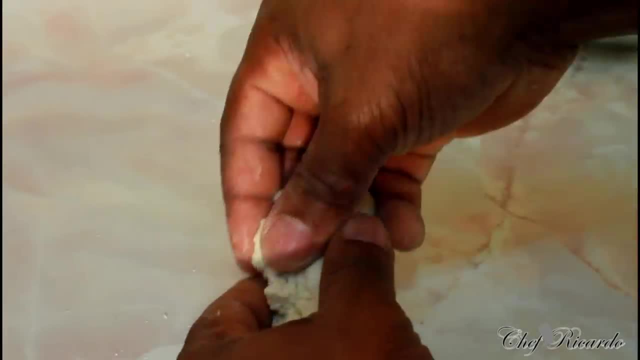 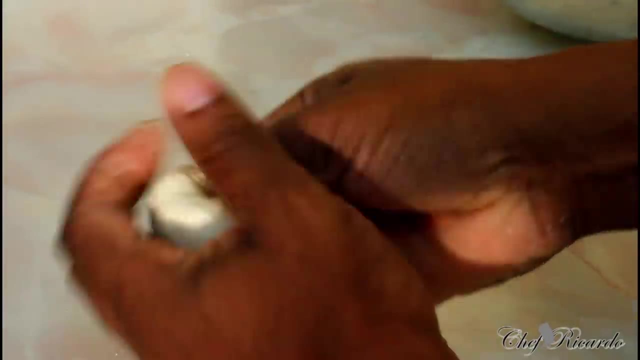 Or you can also do it by breaking off a little piece like this and simple, just fold it into your hand like this, like you are making a big dumpling Boy. is that a big dumpling? it is a mini fried dumpling, this one. 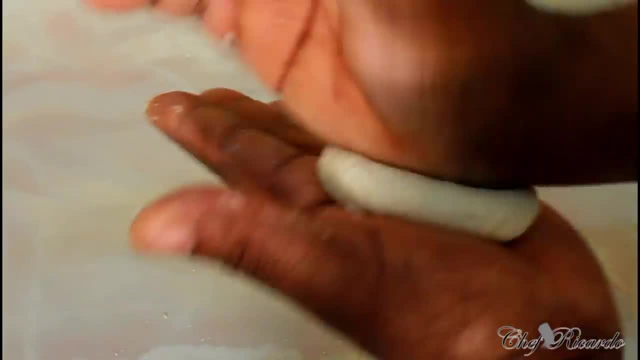 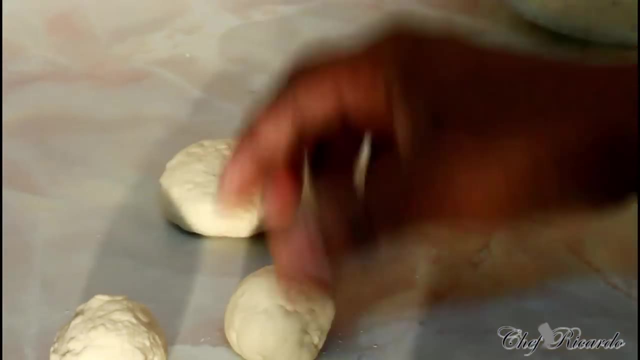 Some people do it this kind of way and press it out inside of their hand. alright, So there is one, two, three, three different kinds of ways where you can do your dumpling right here. guys, This is the three lovely different kinds of ways. 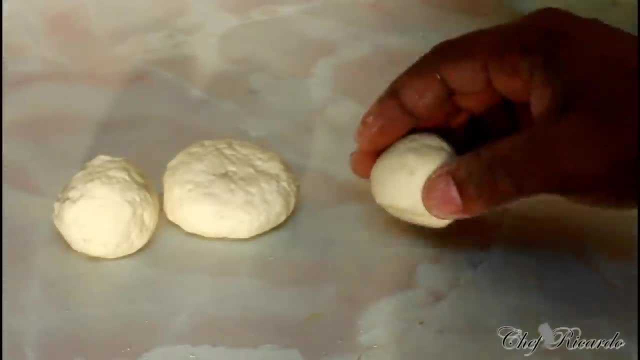 So which one of the ways do you want to do it? Which one of the ways do you want to do it? Which one of the ways? This is up to you. This is your opinion. If you want to roll it, you can roll it. If you want to do it inside of your hand, you can do it inside of your hand. If you want to do it this way, it is up to you. So now, what we are going to do is I will show you how to do your dumpling. 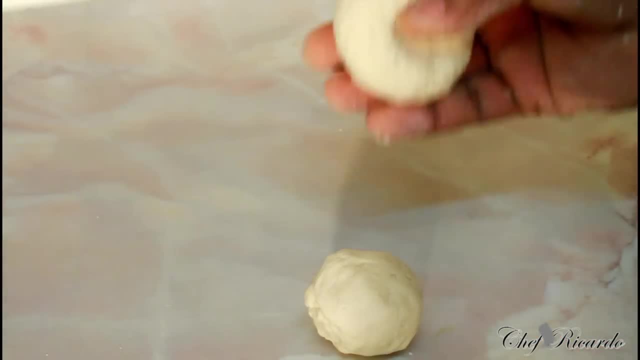 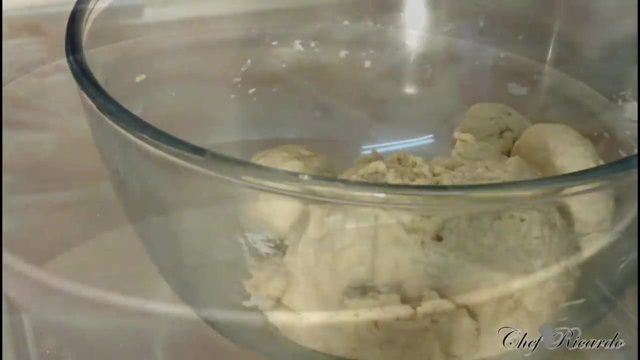 I am going to put the camera straight to the frying pan, alright, And I am going to show you the next level. So, basically, I am going to explain it to you now that inside of this is a lovely, nice, lovely. I have it. 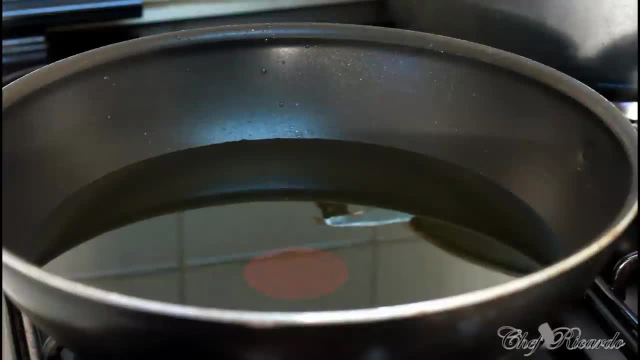 Let's say you are using a pot or a frying pan, yeah, All you need to do is just put probably two and half cups of vegetable oil or olive oil- Whatever oil you want to use- inside of a pot. Make it not too hot, because you don't want your dumpling to really, really burn. 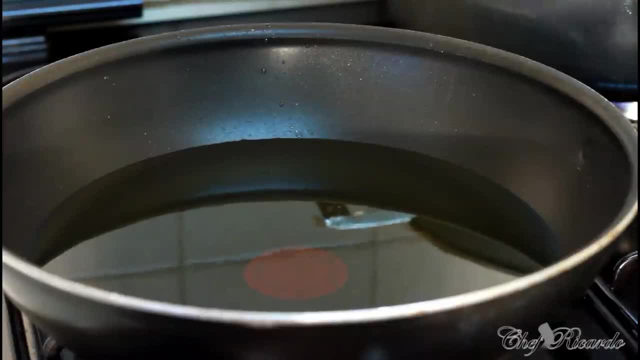 So put it on a medium size heat. but as you can see how much oil you shall have inside of the pot, I did measure it. I just put some oil inside of it So roughly. I am just giving you an advice. you can use two and half cups of vegetable. 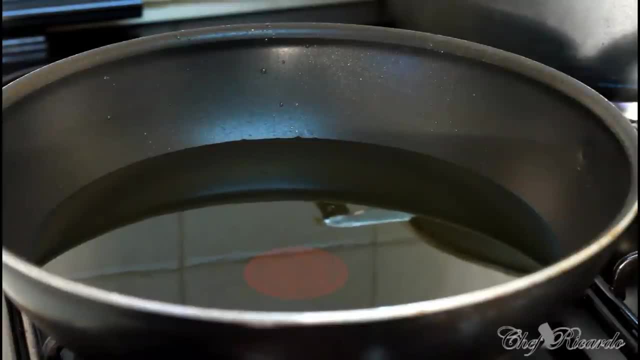 oil or olive oil. alright, right, make it hot, not really too hot for your dumpling to burn up. so basically, let's do one of the dumplings to show you. all right, lovely. so i'm gonna put in this one to see if it's really. 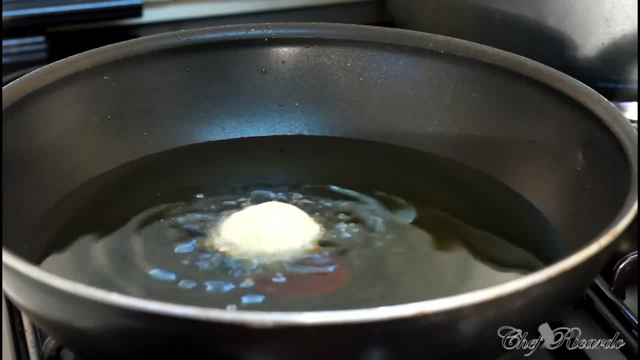 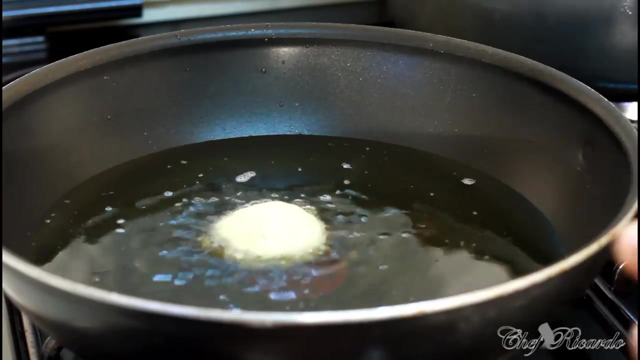 if it's fine. you see, that's what you're gonna looking for. um, sometimes it's good for the aisle to cover the dumpling, but i didn't put a whirlpool eye because i'm not making too much fried dumpling, all right. so, basically, as i can see, that's what you're looking for and i have it. 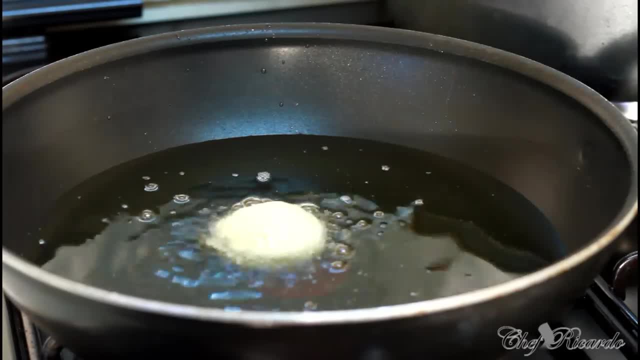 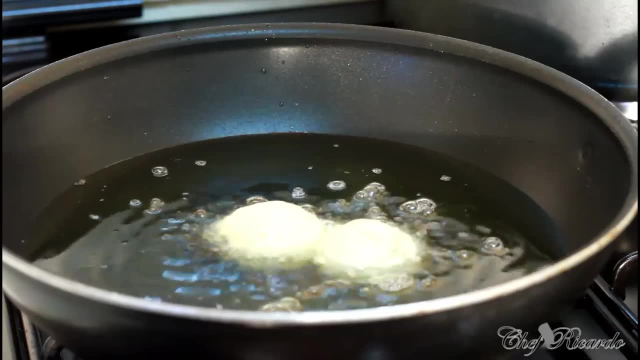 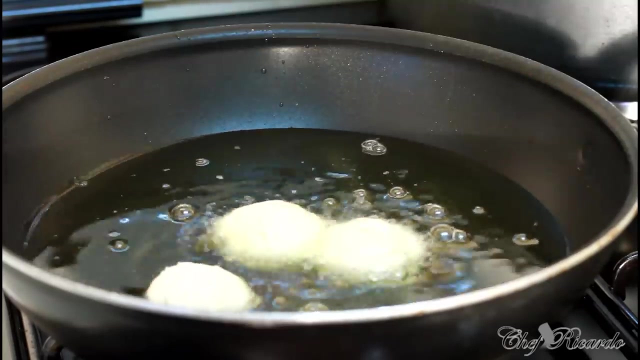 on a medium size eat. you don't want it too high guys. so i'm gonna simple flip this part with some fried dumpling and i'm gonna make them not too big- very small as you can see- and i'm rolling them on my surface because for me it's a little bit more easier for rolling on the surface. 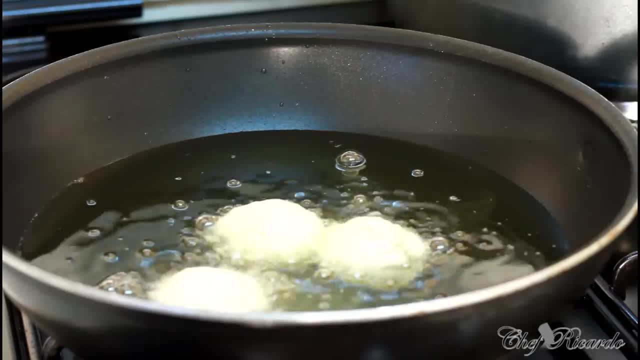 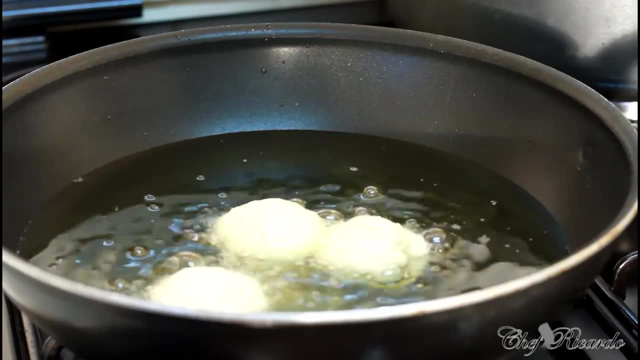 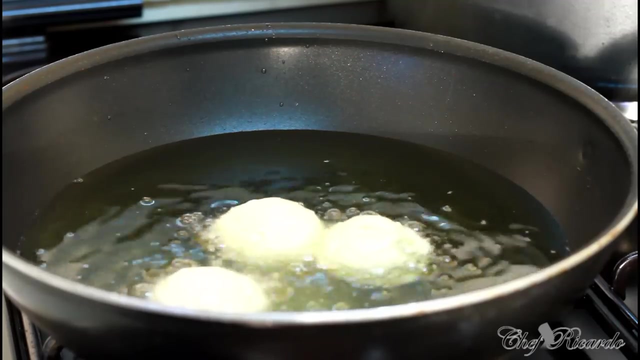 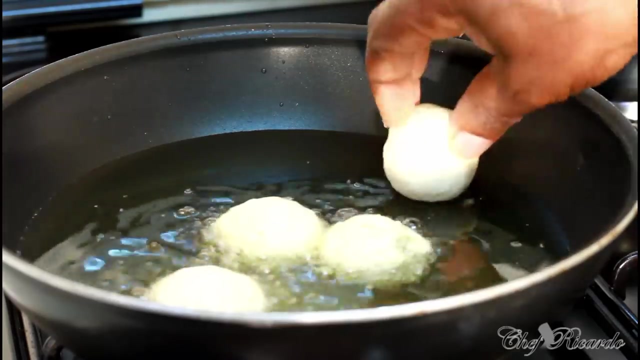 and i'm gonna make their fry for roughly about every time i'm gonna, once you get that lovely brown, goldish color, what you're looking for. so basically, i might make their fries roughly about seven minutes on each side until they get that lovely brown color. all right, so this i'm gonna fill it up with some fried dumplings. 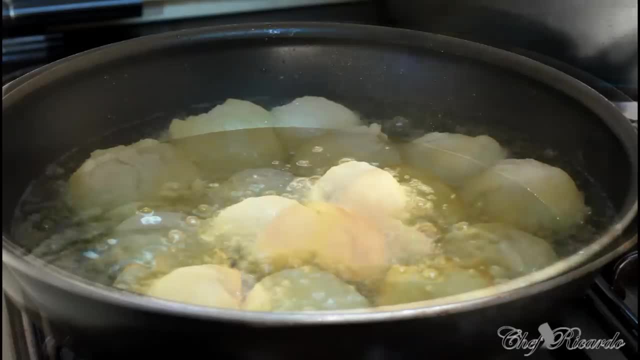 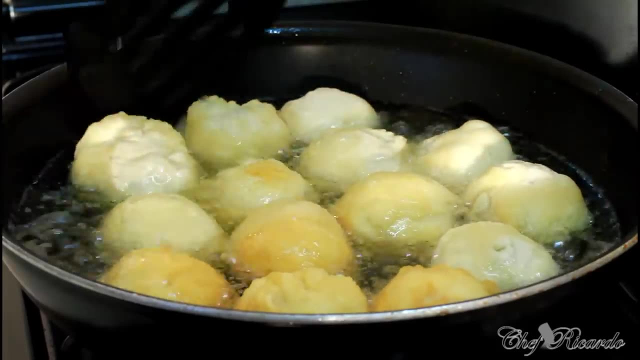 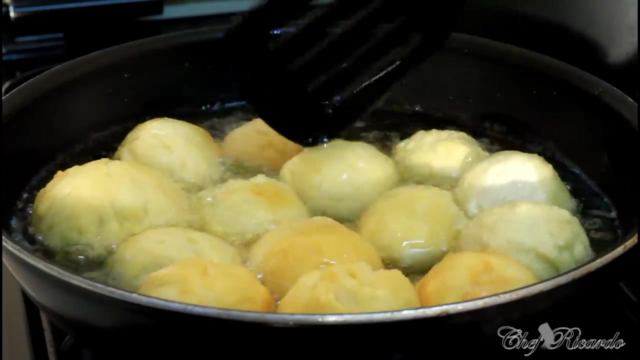 guys. i love this, as you can see exactly where chef ricotta is all about: the fried dumpling right here, guys. so hopefully you guys can do this at home very easy and simple for your holiday, or for your husband or for your kids, them and, as you can see, just like that, very easy and 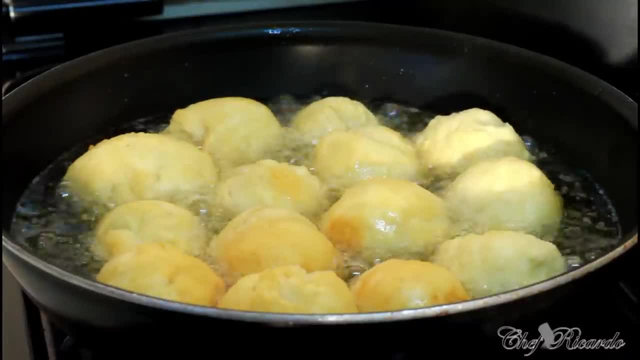 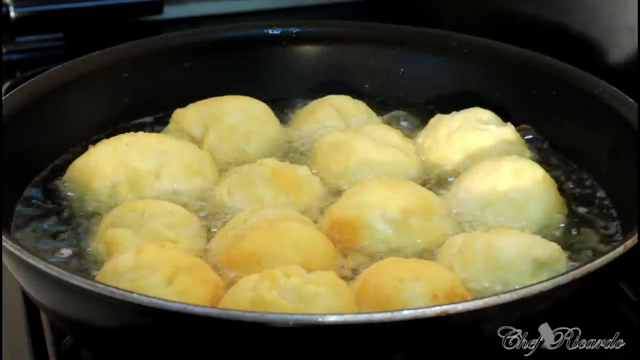 simple guys. hopefully it will be a benefit to you, and this is from chef ricotta and the team. so, basically, as you can see, i'm making them get that lovely, lovely fry which i'm looking for, that goldish color looking nice so far. so, as you can see, i got a medium size eat. 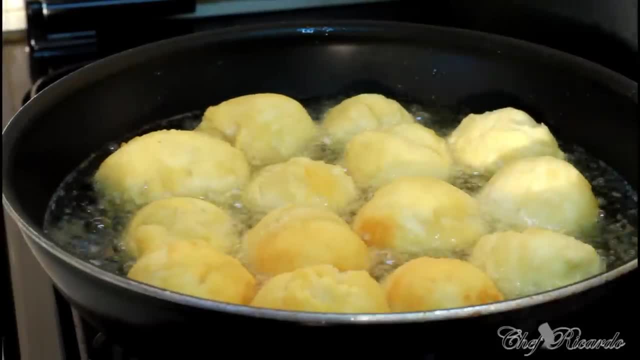 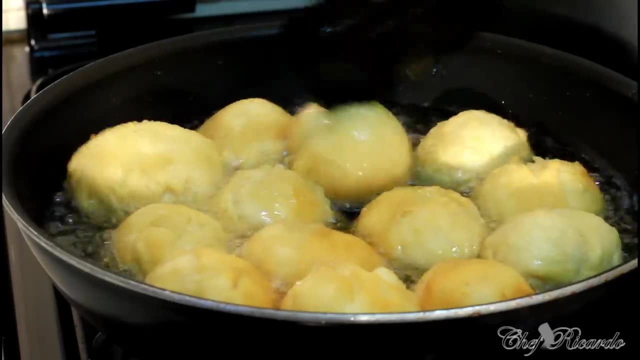 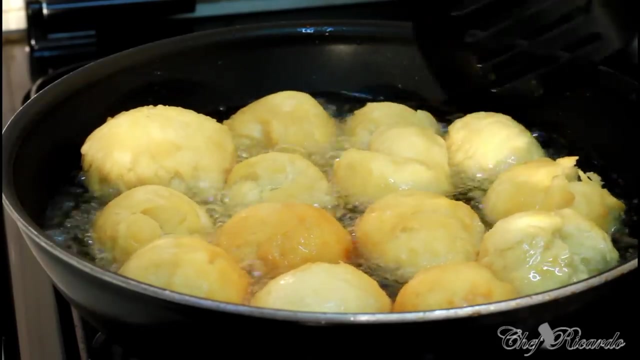 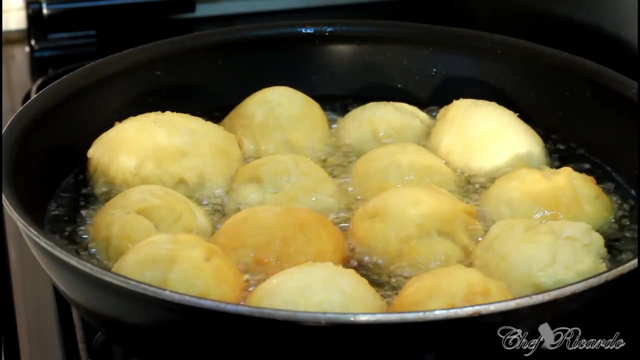 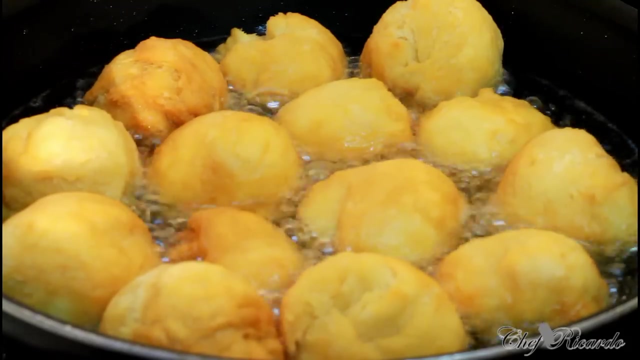 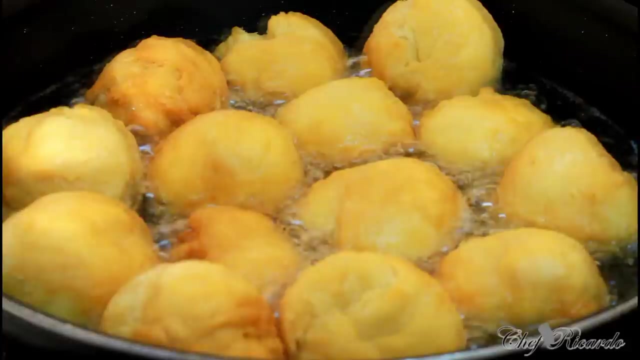 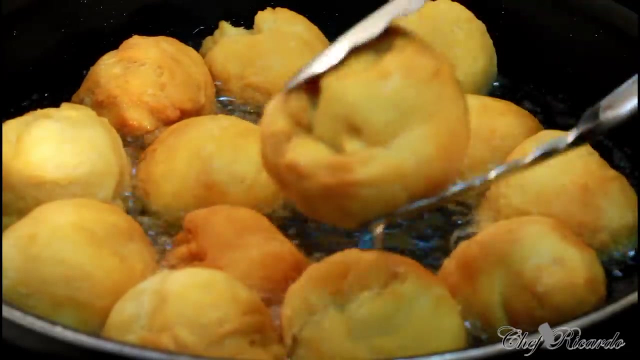 and i'm not rushing it to fry so you can see looking lovely and nice and i'm going to just so: yummy, lovely, lovely color. this is a color which I'm looking for, a lovely brown, goldish color that's beautiful. so basically we need to do is just get a. 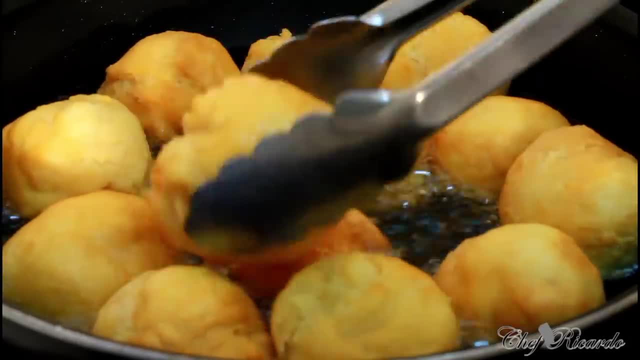 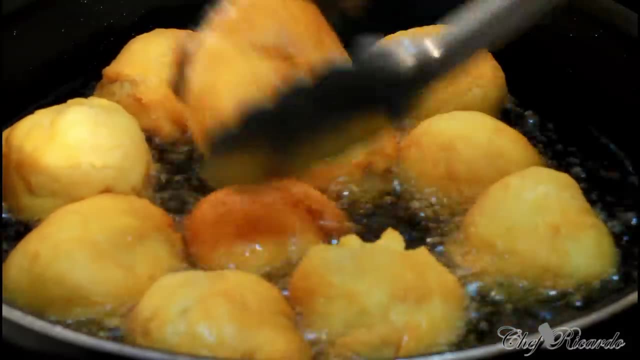 piece of a napkin and put them in on it to get rid of the grease. but I will show you the next section which I'm talking about when they get to that level. but as you can see, he's looking so fantastic guys. the recipe is very easy.